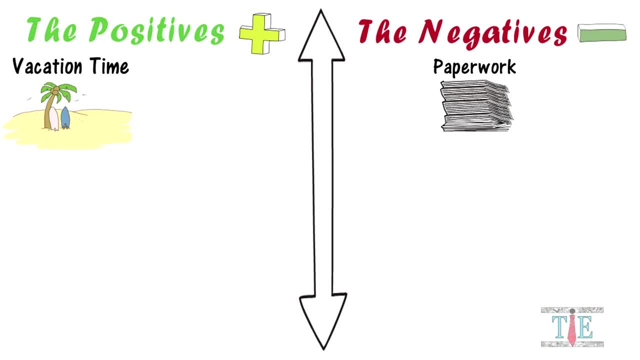 tests and quizzes isn't fun at all. Then comes the lesson planning and data tracking. All I have to say is three o'clock. Teachers get out of work at three o'clock, which usually avoids traffic And gets teachers home in time to see their children. The teaching profession is not one. 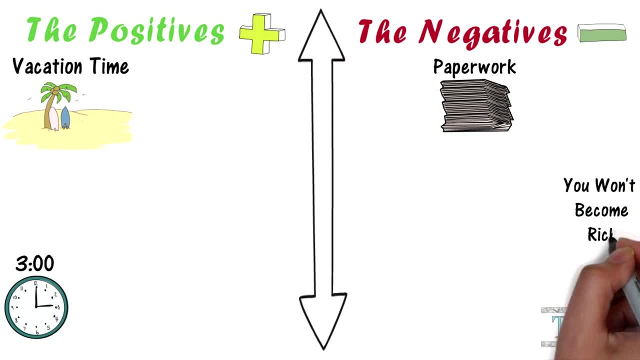 where you're going to become rich. Everyone seems to know that teachers don't make much money. Nevertheless, many teachers are forced to work a second and third job just to pay the bills. Not having financial security is a tough way to live Now, although you won't get rich as a teacher. 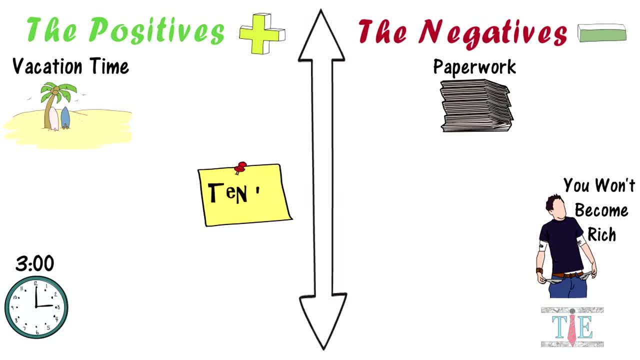 it is a very stable and secure job. Tenure is a special security afforded to teachers. Another negative of teaching is having to prepare students for standardized tests. Today, teachers are held responsible through standardized testing, which is a great deal of pressure Teachers get to make use of. 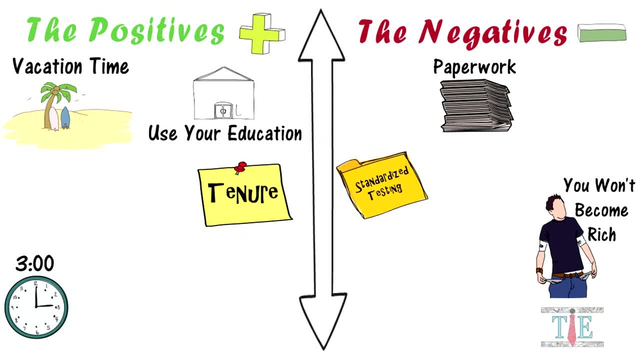 their education. Many people go to college and don't do anything with their degree. They find different lines of work. Teachers, however, pass what they've learned on to others. Most jobs don't require you to bring your work home with you. Teachers will tell you that they. 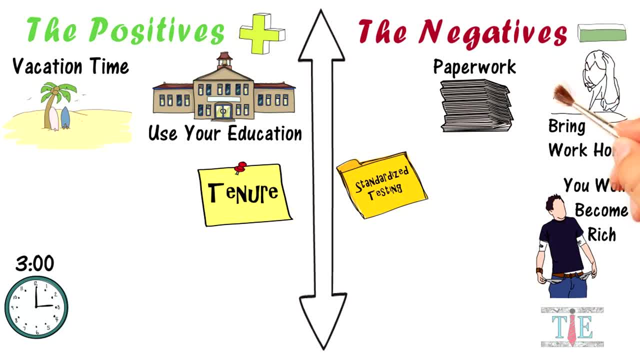 are spending more and more time working at home. They are responsible for the work that they do. They are responding to emails, lesson planning, giving attention etc. and so forth. Forming relationships with your co-workers is what I enjoy most, So I'll give a quick shout out to Mansfield Dr. 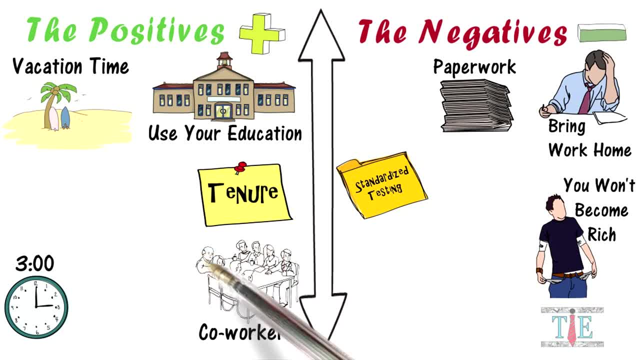 Helfand, Gabe's, Trek Subula, everybody that I've met, and I'm sure, as a teacher, you'll make some great connections as well. One of the toughest situations is teaching emotionally and behavioral students. Some students can be really aggressive, hurtful and outright dangerous. Yes, they are only children and we care about them. 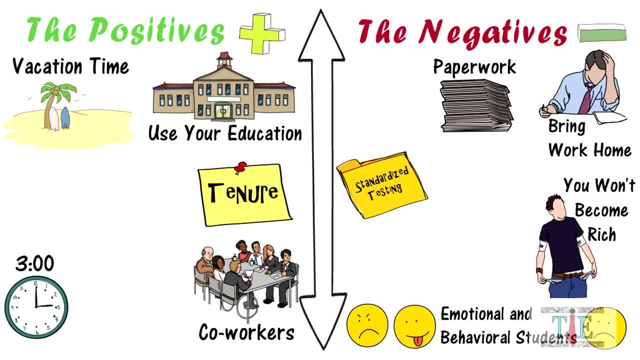 but they can still create pain and misery to a teacher. The best reason for being a teacher is that you get to be a hero to some of your students. In this job, you can actually make a difference in the lives of your students, which is an amazing feeling. 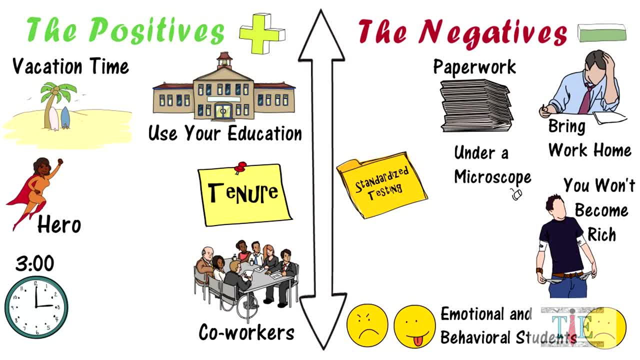 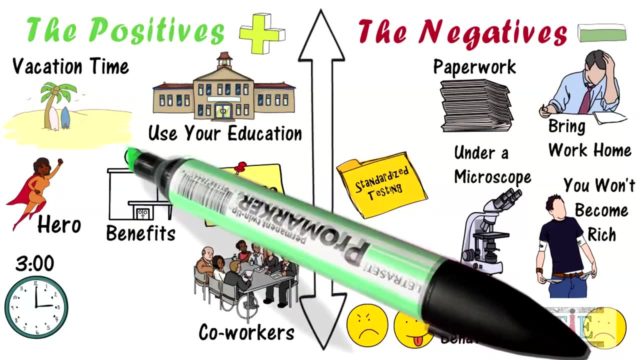 One of the bad things about being a teacher is that you are under a microscope and held to a higher standard. One of the more practical reasons to become a teacher is the benefits that come with the job. Teaching jobs come with medical and dental benefits.